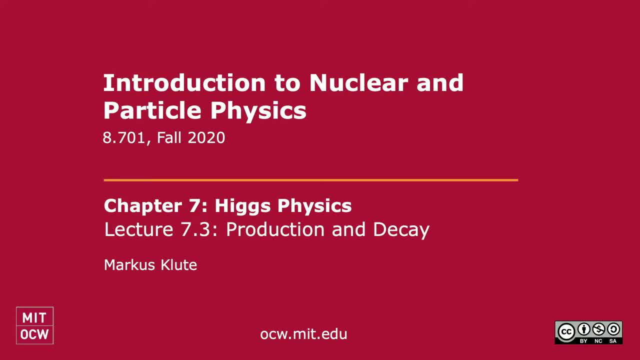 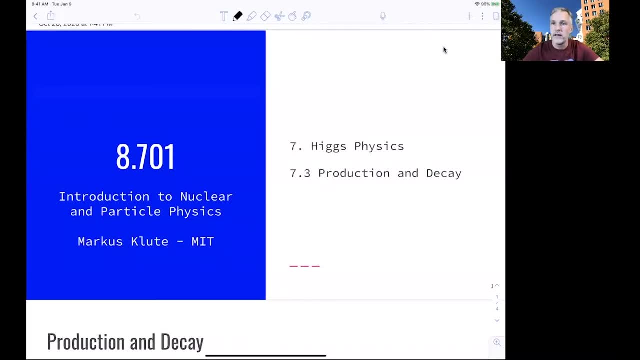 Welcome back to H701.. So now, the theory about Higgs boson is quite interesting, and we have seen that it's able to produce masses of boson, the nephromions. But you know, as Feynman said, a theory is only as good as the experiment. And so you know, we have to actually find Higgs bosons. 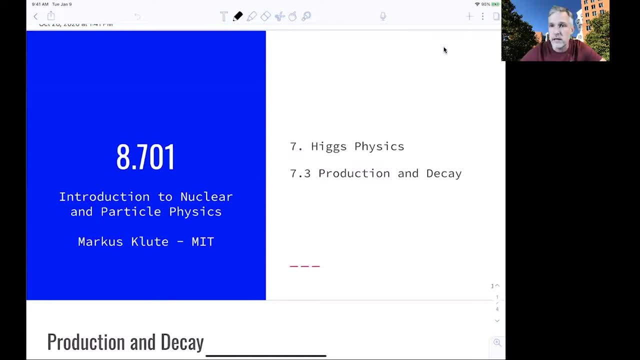 and measure their properties and see whether or not their properties are consistent with the standard model, And so the first question we have to ask is: how are Higgs bosons actually produced and how they might decay? So this little video is just talking about this in very simple terms. 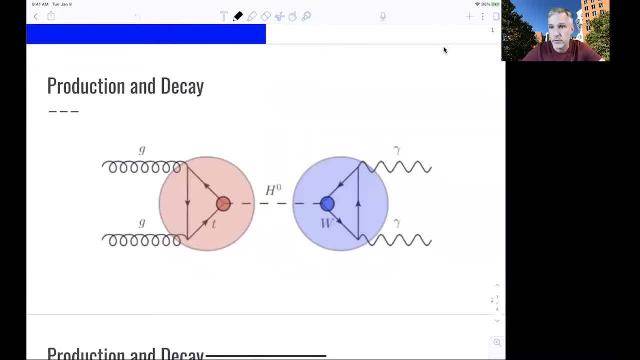 So we are able to produce Higgs bosons at proton-proton machines or proton-proton colliders, Because they are able to bring collisions or produce collisions which allow to have energies of a mass scale consistent with the Higgs boson. You already know now that the Higgs boson has a 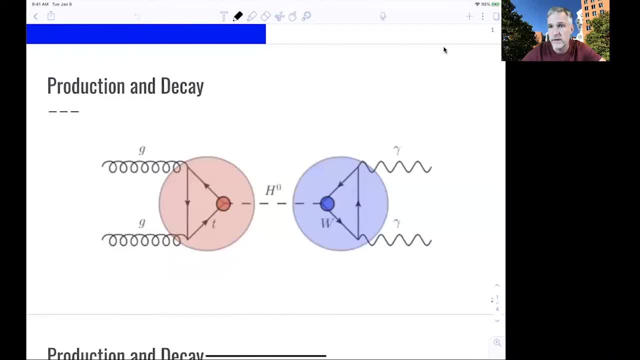 mass of 125 GV, So the collisions have to have enough energy to produce this particle. We're using protons to do this, because protons can be accelerated easier than leptons, for example, to those energies. But protons themselves are, as we have seen, objects which consist of quarks and gluons. So how do gluons now produce Higgs bosons? 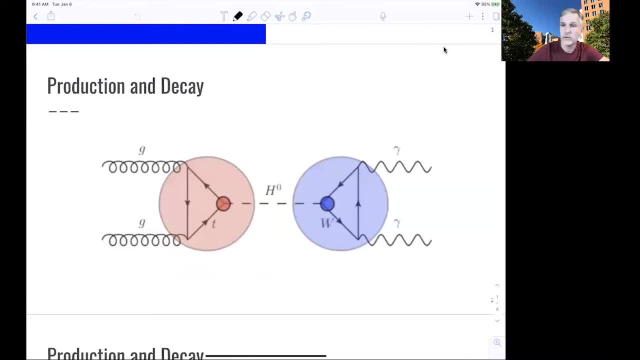 And this is shown in this Feynman diagram here, where you have two gluons from two colliding protons and they are able, via this loop diagram, triangle diagram, including a top quark- top quark goes around here- to cause an excitation in the vacuum, which is the Higgs boson. 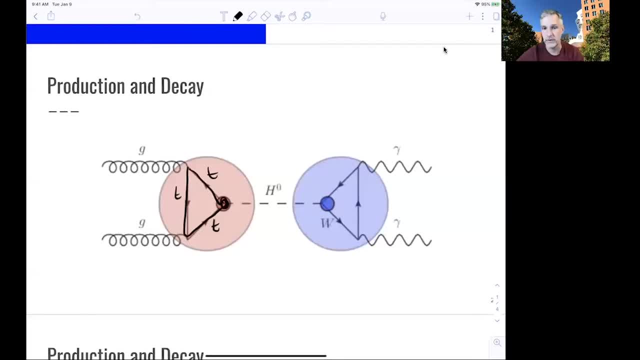 They couple to the vacuum, producing the Higgs boson, And then instantaneously the Higgs boson decays. and it can do this in various ways and we'll look at this on the next slide. And in this example it decays via a similar triangle, loop into a W Right, And then the W is electrically charged. 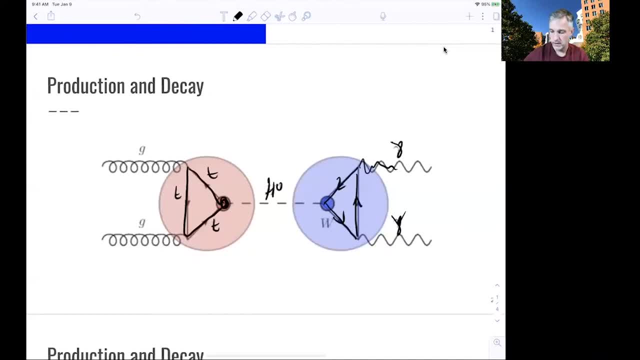 and can radiate a pair of photons. So, while the gluons and the photons are massless, we are able to produce Higgs bosons, where the solutions of two gluons, and observe it via decay into photons. This is quite spectacular. In more general ways, it's not just one mechanism to produce Higgs bosons, but there are various. 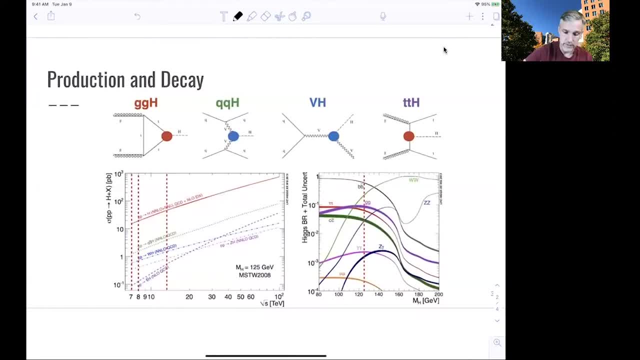 And the leading ones are shown here. We have just looked at this first one, which is called gluon fusion channel. So two gluons fuse together to an Higgs Boson. There's this one here. the second one, which is called vector boson fusion, 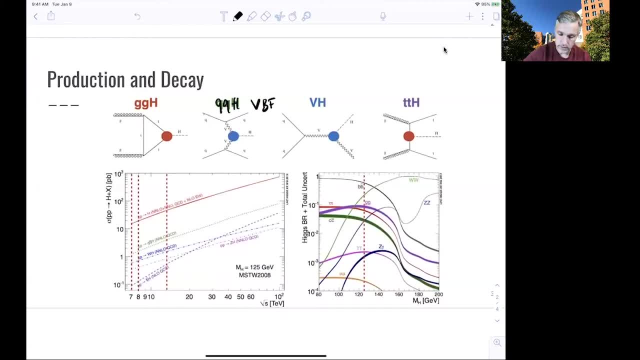 VBF, where we have the quarks radiate, two vector bosons- This is either the Z boson or the W boson- And then those couple to the Higgs field and produce the Higgs boson. We can also have associated production. 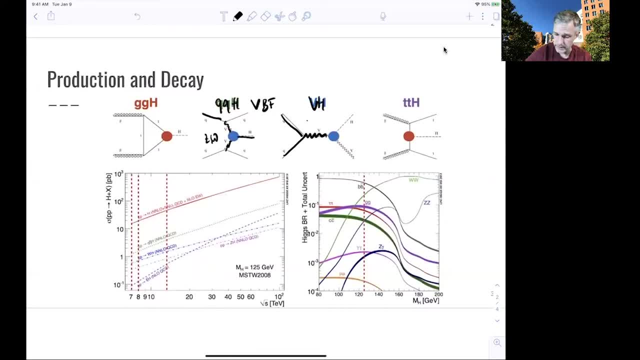 where we have two quarks, via again a Z boson or a W boson, radiating then a Z boson or W boson and generating a Higgs. And then a very exciting one is the last one here- where the Higgs boson is produced in association. 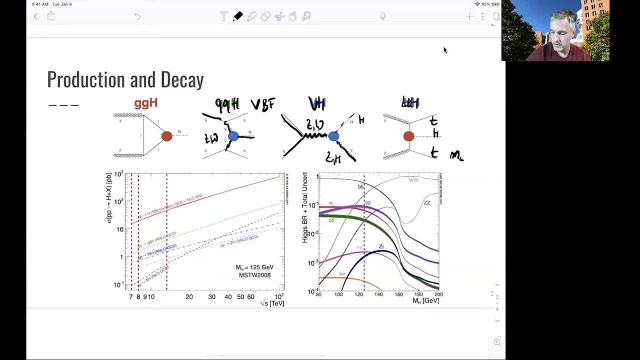 with two top quarks. Remember, the top quark here has a mass of 175 GeV. The mass of the Higgs boson is 125 GeV, And so we have two of those, So the scale of this event is in the order of 500 GeV. 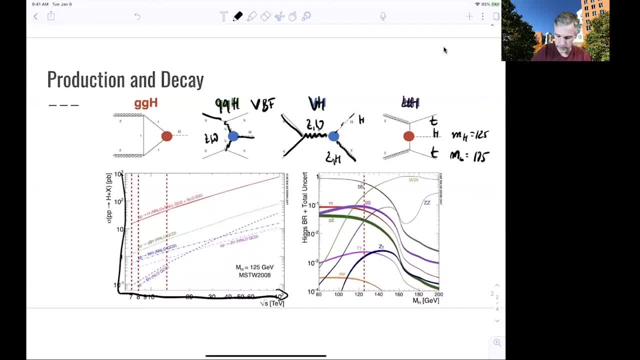 This plot here shows the production cross-section, This function of center of mass energy. Now, the Large Hadron Collider, the LHC, operates currently at 13 GeV. So the cross-section we want to look at are those. So you see that the leading cross-section, which 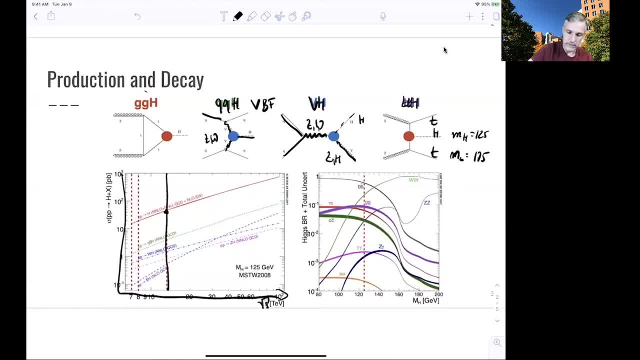 is in the order of tens. of picobahn is the one where we have gluon fusion An order of magnitude less, is the one with vector boson fusion, And then we have associated production, And then the last one is the one where 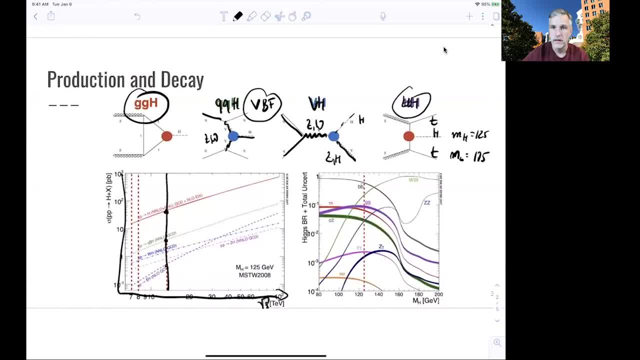 we have fixed bosons produced in association with top quarks. Because the mass scale is much higher, the cross-section for TT Higgs is lower If you increase the center, if you were to increase the center of mass energy of the LHC. 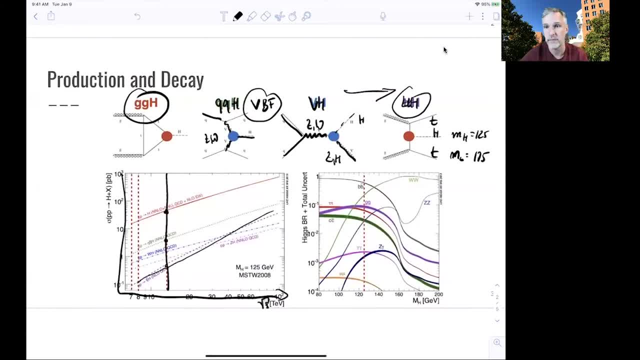 you see this rapid increase in cross-section. It's just because there is more phase space available for this production. The coupling here and the coupling here is the same. Then the Higgs boson, as I said, decays, And we have already discussed Higgs- Branschen ratios. 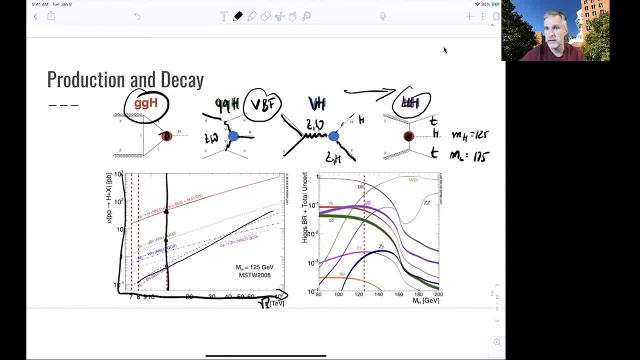 or Branschen ratios in general. And since the coupling of the Higgs boson to fermion is proportional to the mass of the fermions, you see the dominant decay is the one into Higgs to BB bar, And then you can find lower decays to the taus, to charm. 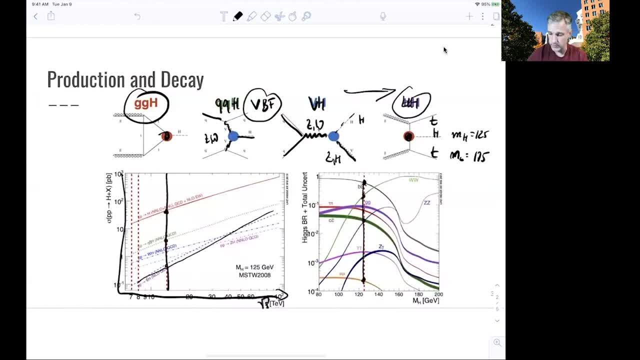 and to muons. here You also have decays into the vector bosons WW and ZZ And so similar triangle diagrams. you have decays into glu-glu and into two-photon as well. So we have already measured the Higgs boson at 125 GeV. 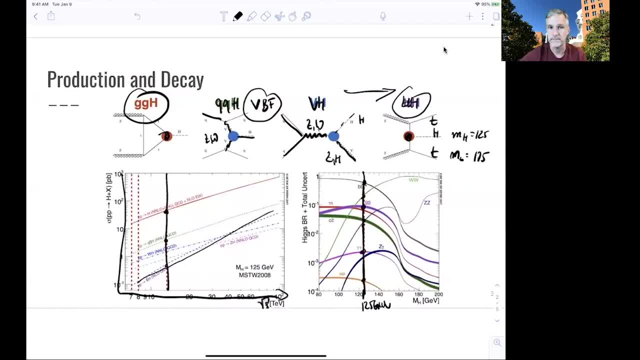 And so those are the Branschen ratios as predicted in the standard model. 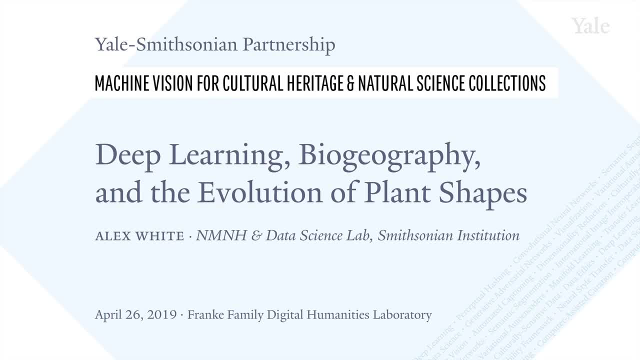 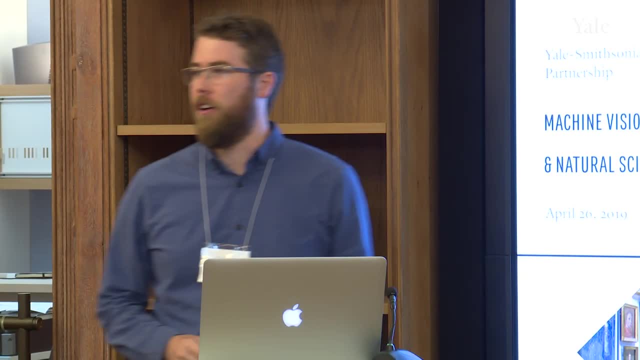 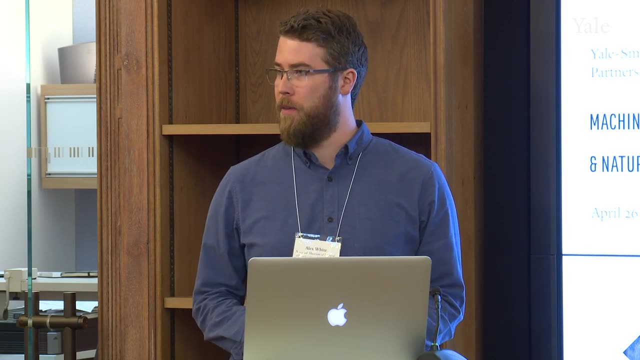 Okay, very excited to be here today to talk to you about work that I've been doing as a postdoc on the evolution of plant shapes using these models that we've been hearing a lot about this morning, So I think there was a good primer for the work that I'm going.